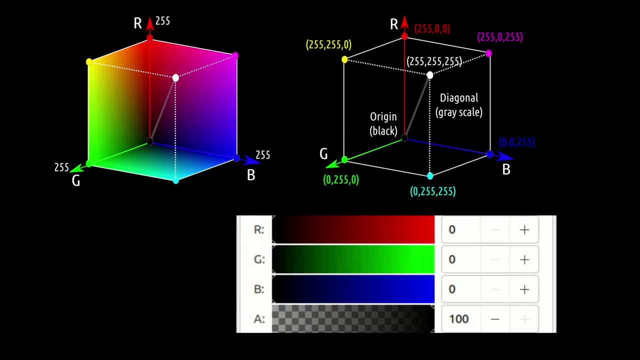 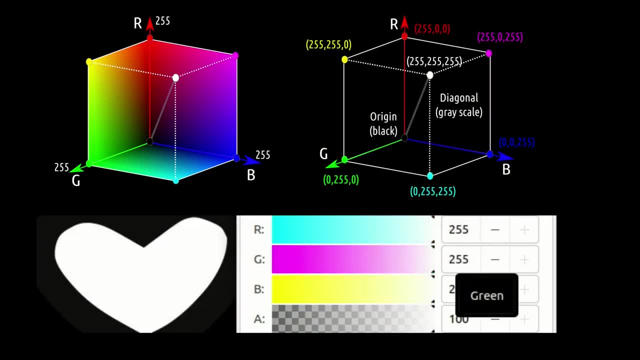 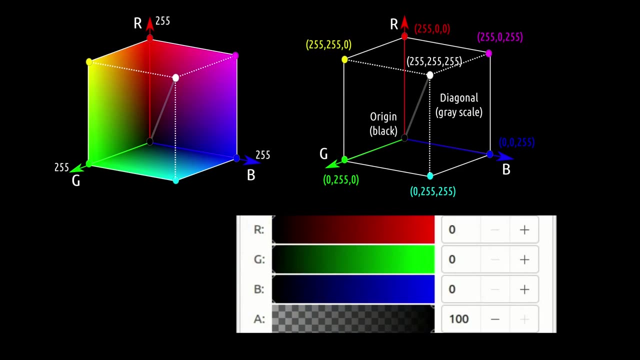 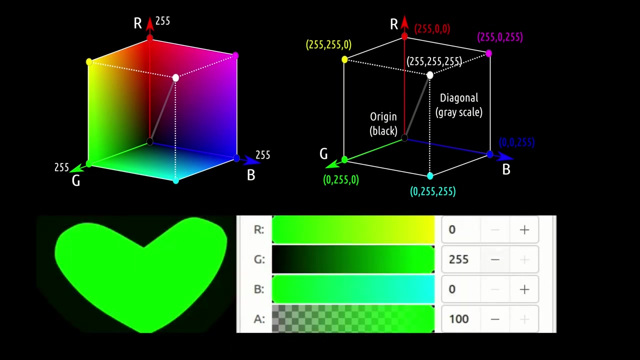 with one axis for each color channel: red, green and blue. The origin of the cube represents the black color and the opposite vertex represents the white color. The diagonal formed by these two vertices corresponds to a gray scale. The other vertices of the cube corresponds to red, green, blue, yellow, magenta and cyan colors. 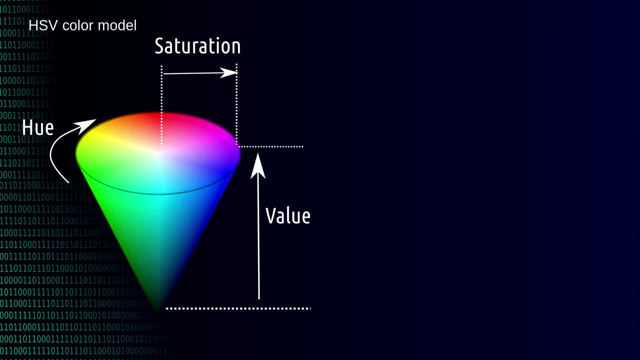 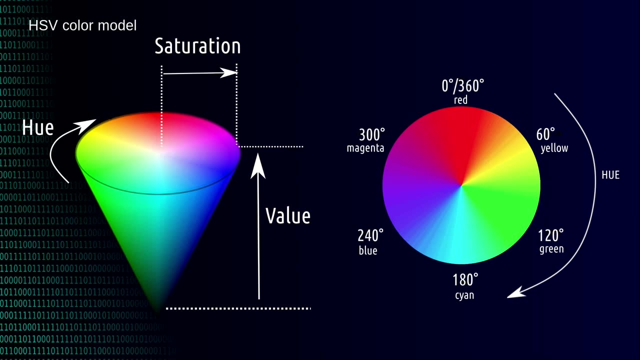 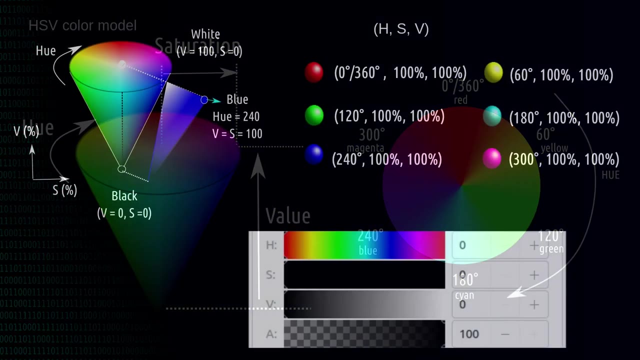 The HSV module is an alternative representation of the RGB color module. In this module, the colors are differentiated according to the hue, saturation and value. The color hue varies from 0 to 360 degrees. The black and white colors are independent of the hue. 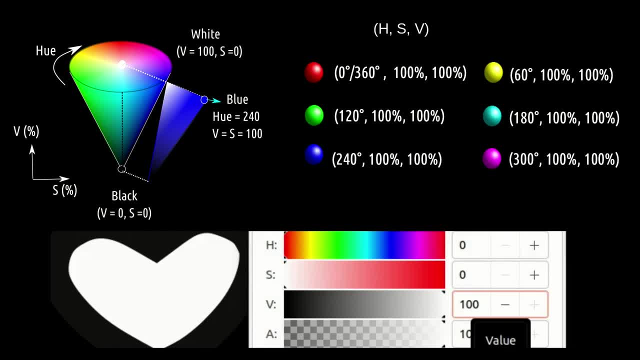 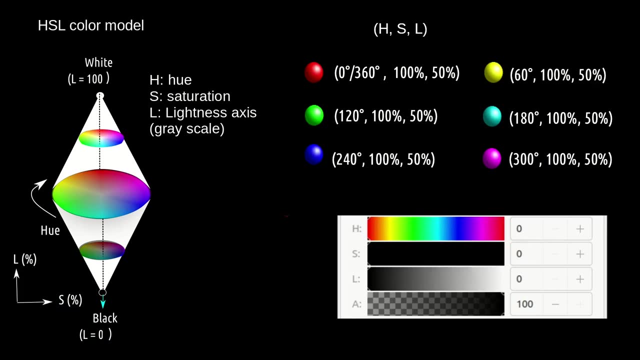 White color has 100% value and no saturation, while the black color has no value or saturation. All pure colors and their combinations have 100% of saturation and value. The HSL module is an alternative representation of the RGB color module In this module. 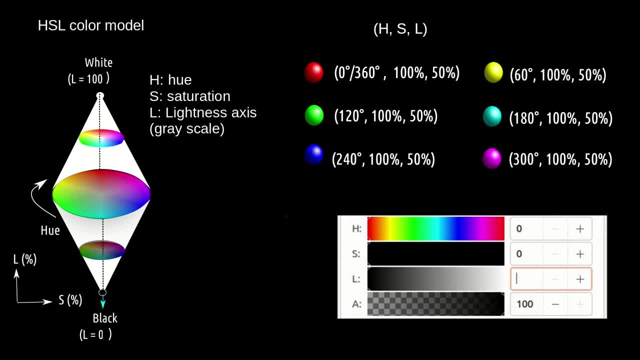 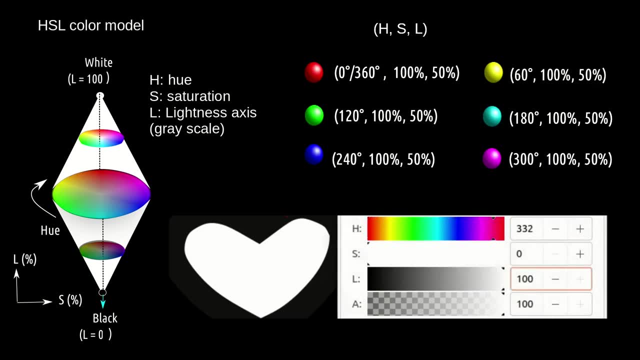 the colors are differentiated based on hue, saturation and lightness. The white color has 100% of lightness and black color has 0 lightness. Both white and black are independent of hue and saturation, Keeping the saturation equal 0 and changing the lightness. 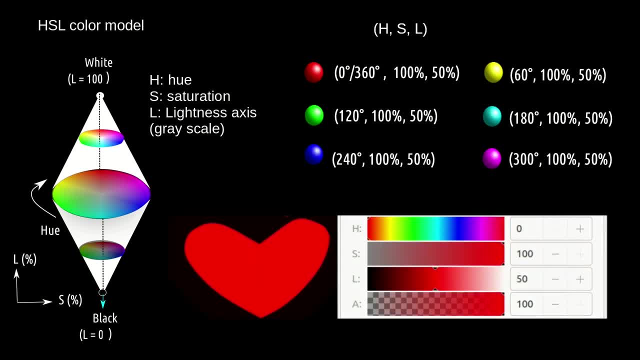 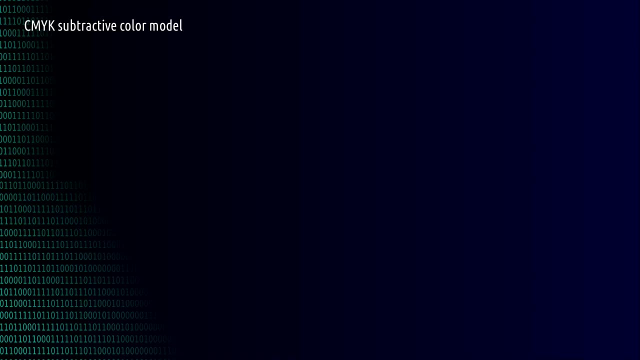 we have the gray scale The pure colors lies at. lightness equals 50% and saturation equals 100%. Unlike the RGB module, the CMYK module is a subtractive color module. CMYK works due to the absorption of light. 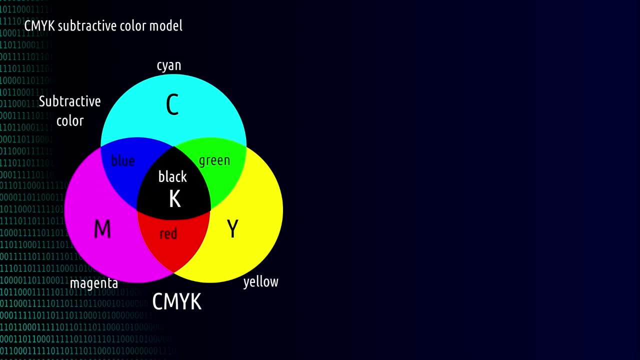 The colors that are seen result from the part of the light that is not absorbed. This module is based on the use of inks, pigments and dyes that absorb color from the white light. The key color is black, which can be obtained by mixing cyan, yellow and magenta inks.